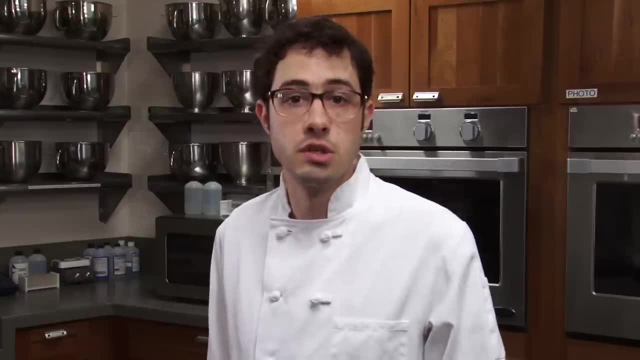 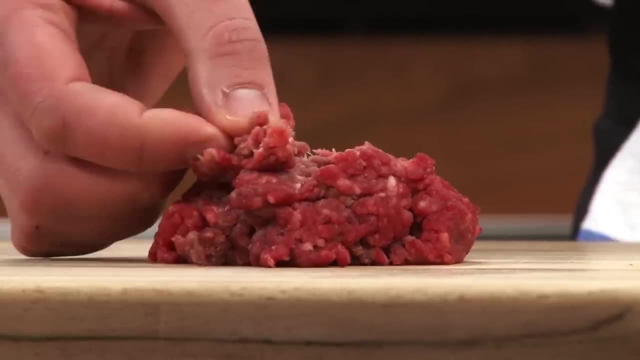 is tough instead of tender, And here's one of the first reasons that you really want to grind your own meat at home. Here I have a pile of store-bought ground beef. As you can see, it's very finely ground. It's sticky and pasty. In addition, it comes very firmly packed in the package. So 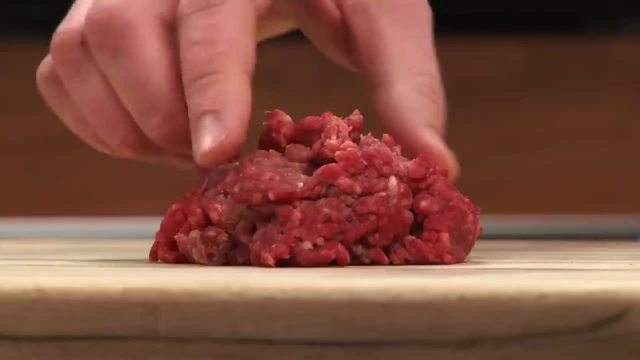 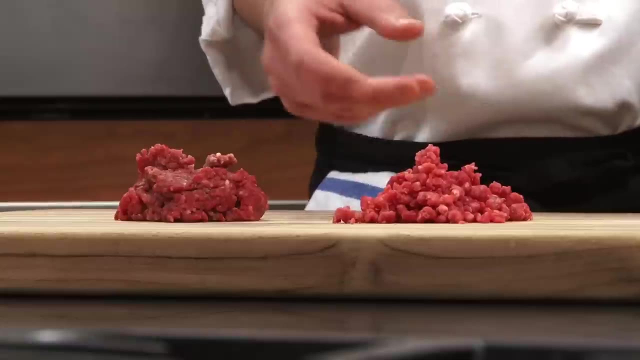 what you end up with is tough, dense burgers with a mealy texture. You really have no idea what exactly is going into your ground beef blend. It could be from many different cuts and even different cows. For comparison, I have a pile of beef that we ground here in. 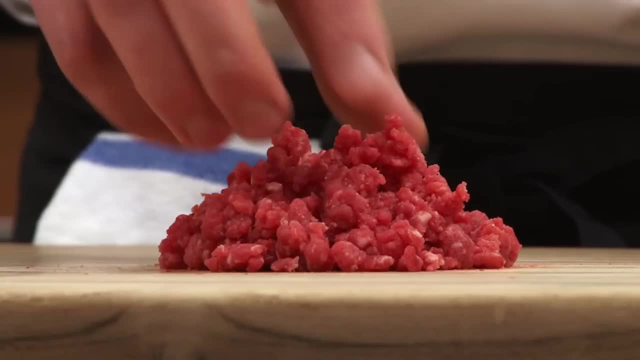 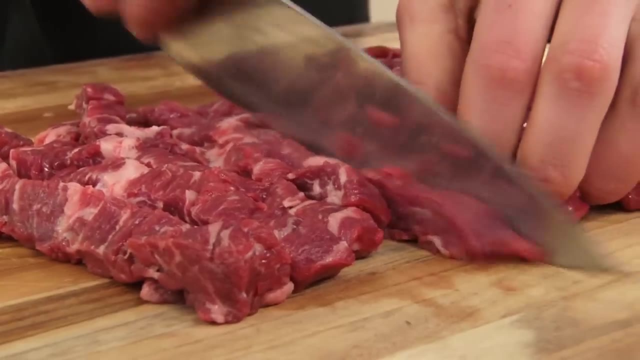 the test kitchen using nothing more than our freezer and a food processor. Now, as you can see, it crumbles through my fingers, has a very loose texture and it's going to cook up into a burger with a loose, crumbly texture. In addition, because we choose the 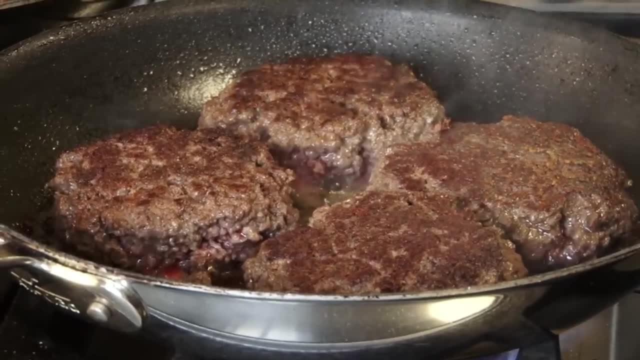 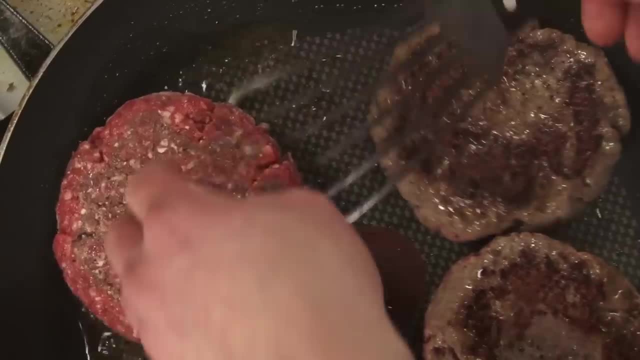 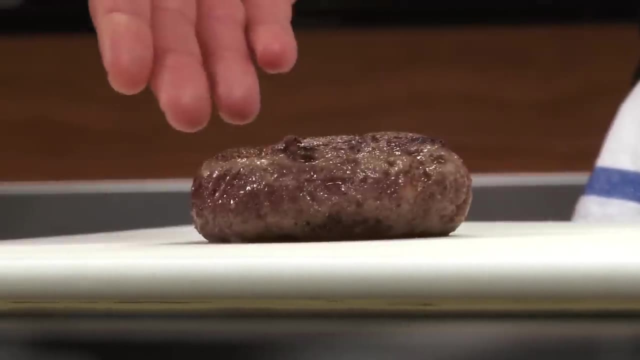 So now for the fun part. Our taste test showed that burgers made with home ground beef were indeed more tender than those with store-bought. But we wanted a way to show it, So I've cooked off two burgers, one with home ground beef and the other with store-bought. Both weighed. 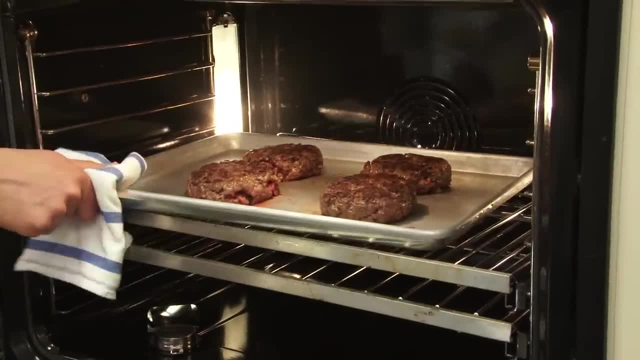 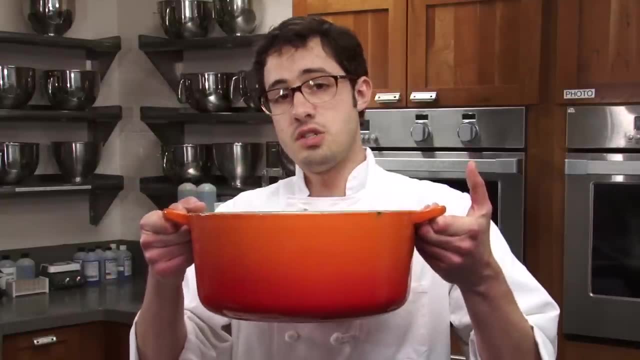 eight ounces raw. I seared both on both sides and then transferred them to a 300 degree oven to finish cooking. Now they're both rested for five minutes. I'm going to drop a 10 pound Dutch oven from six inches up on top of both and we'll see how much they splatter Right. 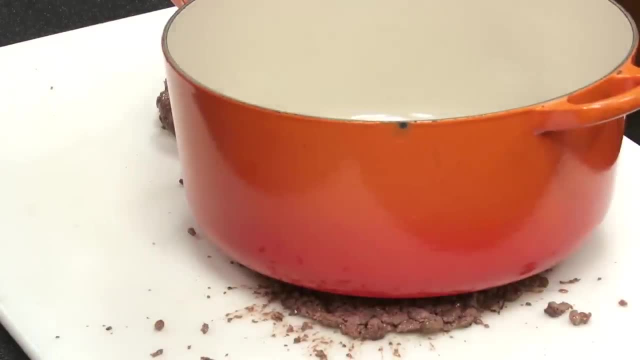 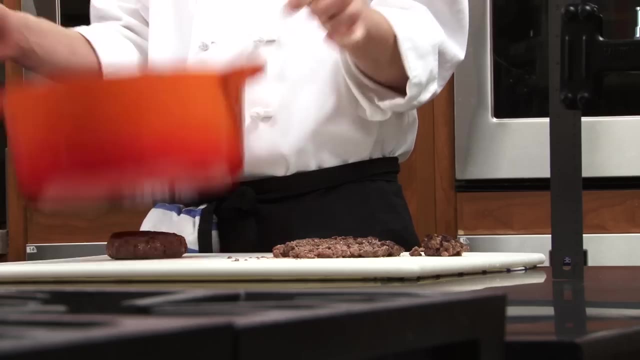 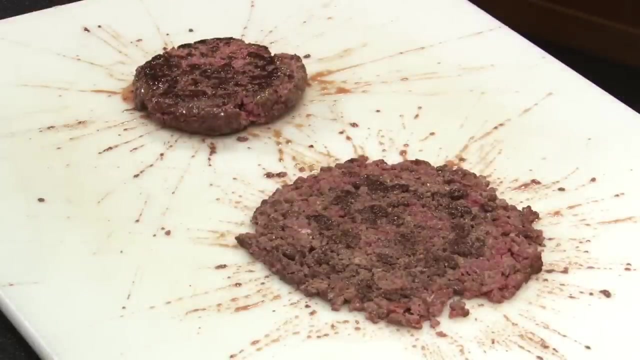 there. All right, All right, ready, Yeah, Does that look good? Yeah, Yeah. Now let's take a look at the aftermath. So you can see there's a pretty dramatic difference. The burger made with store-bought beef is largely intact. 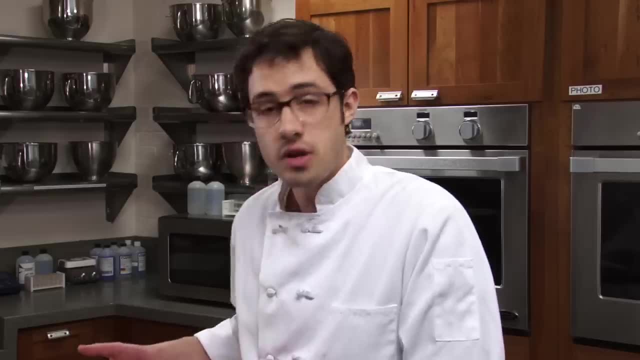 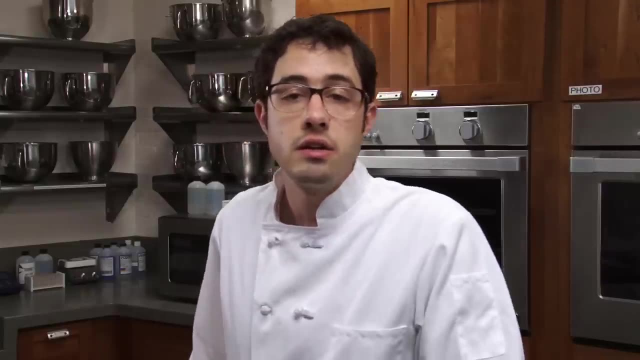 It spilled a little bit of juice, but it didn't really go anywhere on the board. In contrast, the burger made with home-ground beef is completely smashed and flattened Meat flew everywhere. So what can we learn from this? Well, by grinding your own meat at home. 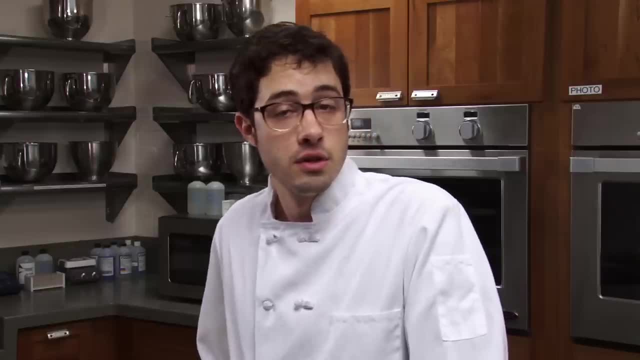 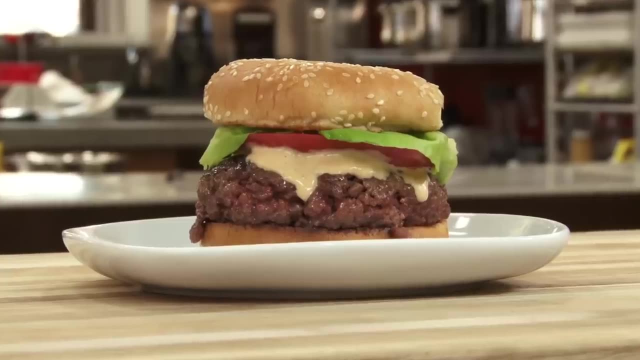 you have control over the cuts that go into it. so you have control over fat and flavor, You have control over the grind size and then how tightly the burger is packed. All of that in the end determines how tender and delicious your burger is.